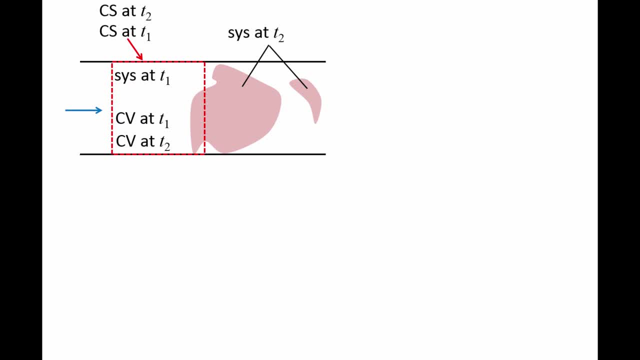 volume and no longer occupy the exact same region of space as the control volume. If we keep track of the pink mass from time t1 to time t2, that is, we are taking the system point of view- the mass at t1 equals the mass at t2.. 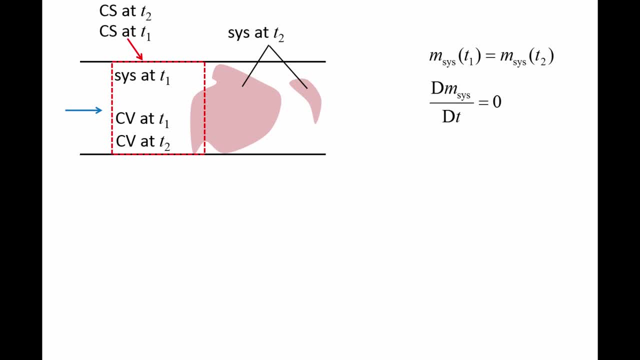 Another way to express this idea mathematically is to say: the time rate of change of the mass in the system is zero. that is, dm. dt equals zero. We will use capital D's in the time derivative to indicate that we are taking the system point of view in describing the conservation of mass. 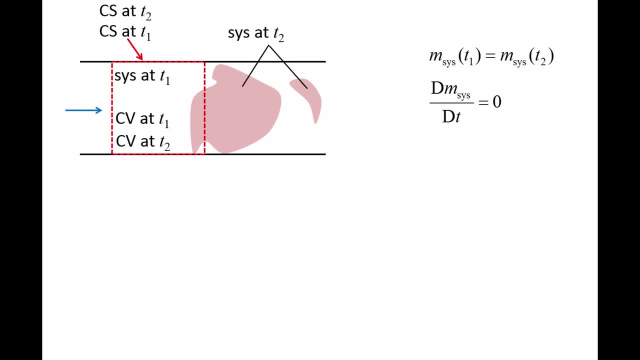 equation. In order to convert the conservation of mass equation for a system to the conservation of mass equation for a control volume, we utilize the Reynolds transport theorem, where the extensive property, capital B, is the mass and the corresponding intensive quantity. lowercase b is 1.. Now plug in the values for capital B and lowercase b. 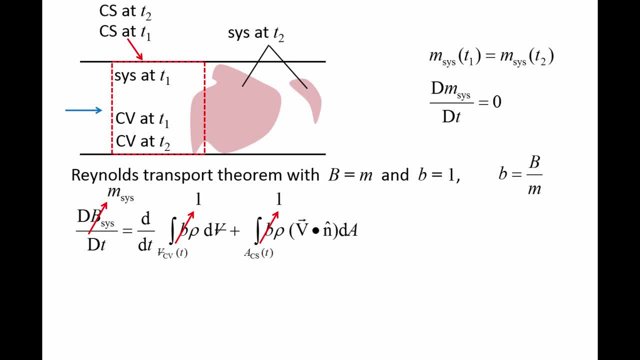 The left side of the equation is the time rate of change of mass in the system point of view, which we have already determined to be zero, and we arrive at the conservation of mass equation for a control volume in its most general form, Zero equals the time derivative of rho dv. 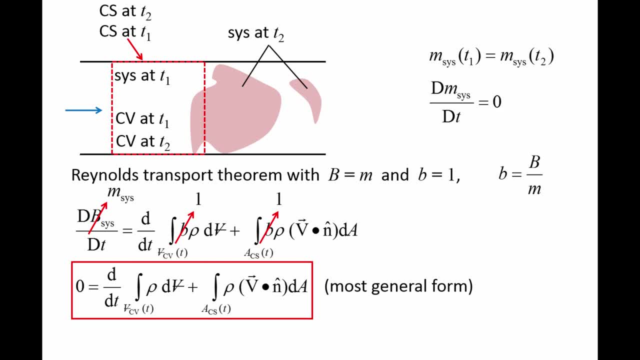 integrated over the entire control volume, plus rho times, the velocity vector, dot n, hat times dA, integrated over the entire control surface. This equation is valid for a control volume that is fixed and rigid, a control volume that is moving at constant velocity. 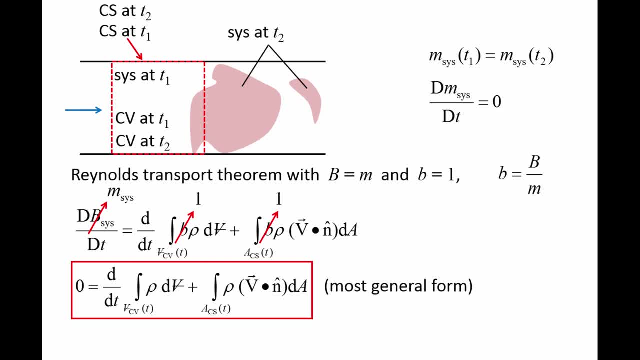 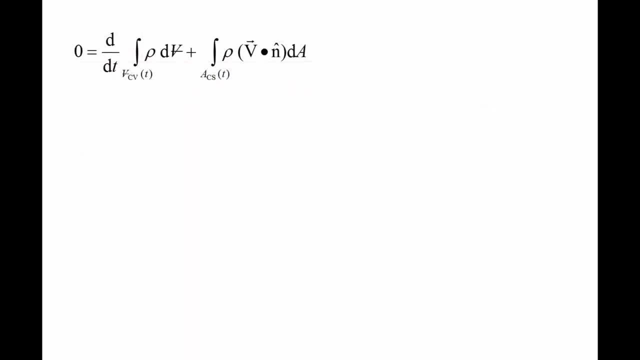 and a control volume that is deforming. It is important to remember that the velocity v is the fluid velocity relative to the control surface. Taking a closer look at this equation, the first term represents the accumulation rate of mass in the control volume, while the second term represents the net mass flux through the control surface. 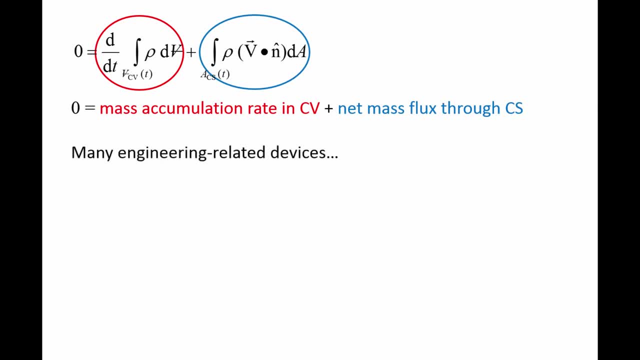 By making a few assumptions, this equation can be greatly simplified and still be useful for a wide variety of engineering-related devices. Most devices, such as pumps, turbines, compressors, pipes and so on, usually operate under steady flow conditions, that is, the flow is constant in time. 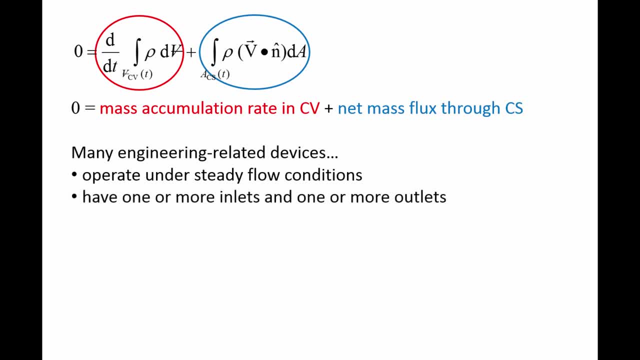 Most devices will have one or more inlets and one or more outlets, And most devices do not deform significantly. For steady flows, the amount of mass in the control volume is constant in time, which means the term with the time derivative is zero, Since the first term is zero. 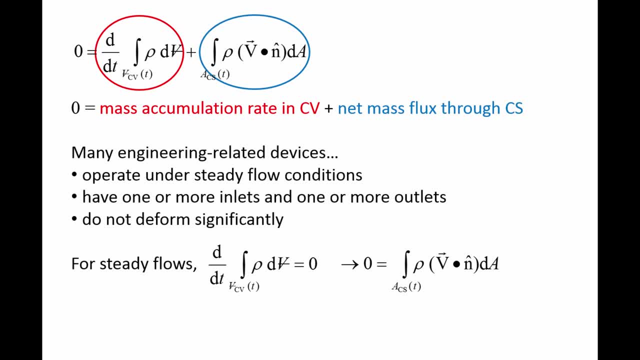 the second term is zero as well. Physically, this means the net mass flux through the control surface is zero. The rate mass enters the control volume is equal to the rate mass leaves the control volume. Now let us look at a generic device which has 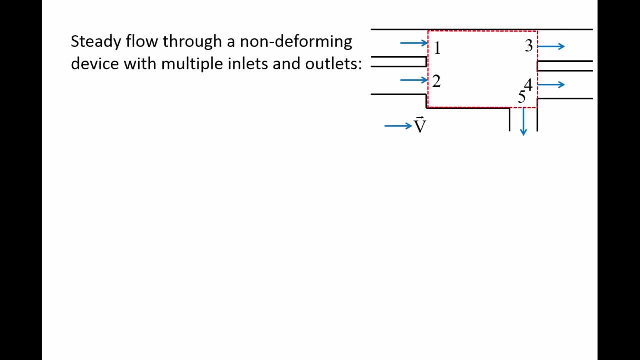 multiple inlets and outlets and does not deform. The device is surrounded by a control surface which is marked by the red dashed lines. The control volume is inside this control surface, The direction of flow is indicated by blue velocity vectors and the inlets are labeled. 1. 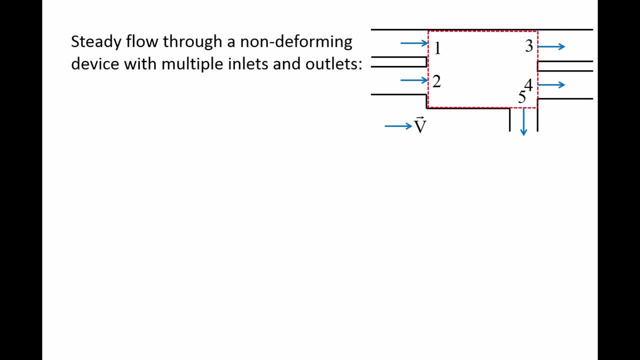 and 2,, while the outlets are labeled 3,, 4, and 5.. The direction of the normal vectors are shown in orange and point outward from the control surface, Since the flow is steady. the surface integral term in the conservation of mass equation- 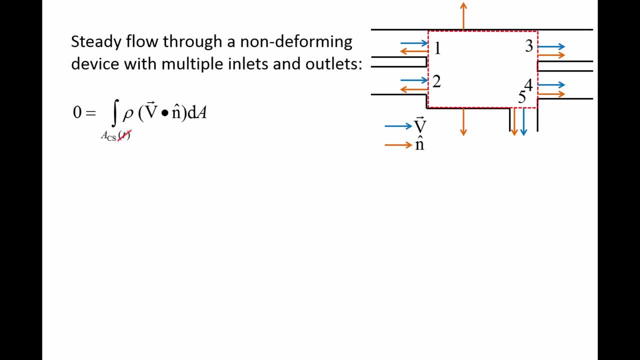 is equal to zero. Also, since the control surface does not change in time, we can remove the time dependence from the limits of integration. Notice that the integral is over the entire control surface. We can break up the control surface into multiple sections and integrate over each of these sections individually. 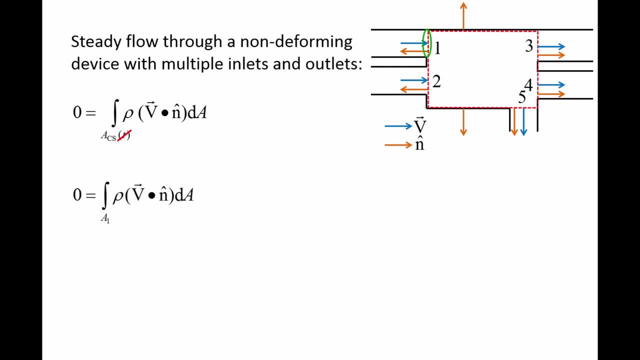 The first integral will cover the area for inlet 1,, the second integral will cover the area for inlet 2,, the third integral will cover the area for outlet 3,, the fourth integral will cover the area for outlet 4, and the fifth integral will cover the area for outlet 5.. We need a sixth. 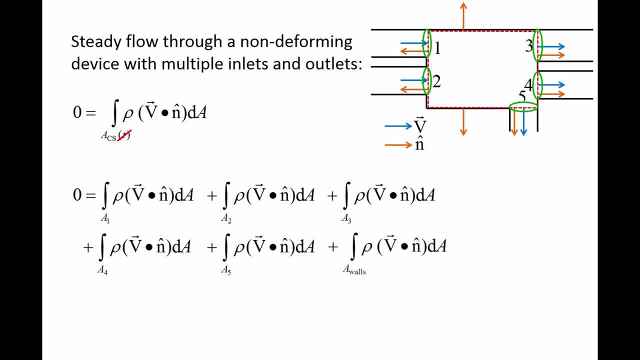 integral to cover the walls of the device. The dot products can be simplified by noticing that the angle between velocity vector and normal vectors are parallel at the inlet and in the the inlets and outlets. Recall that the dot product of any two vectors can be calculated by multiplying the magnitude. 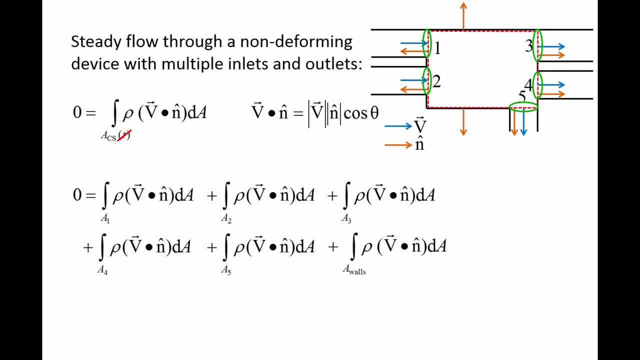 of the two vectors by the cosine of the angle between them. For the inlets, the angle between the velocity vector and normal vector is 180 degrees, which means the dot products for integrals 1 and 2 become negative. v. For the outlets, the angle between the velocity vector and normal vector is 0 degrees, which 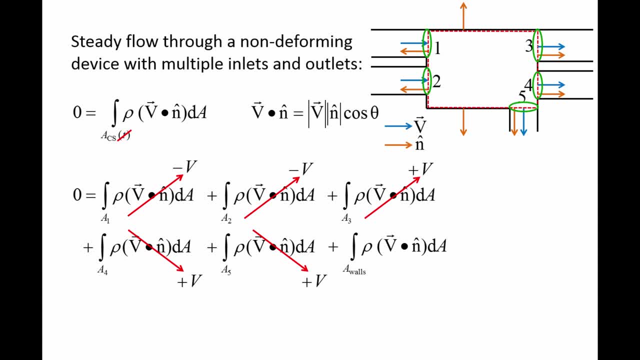 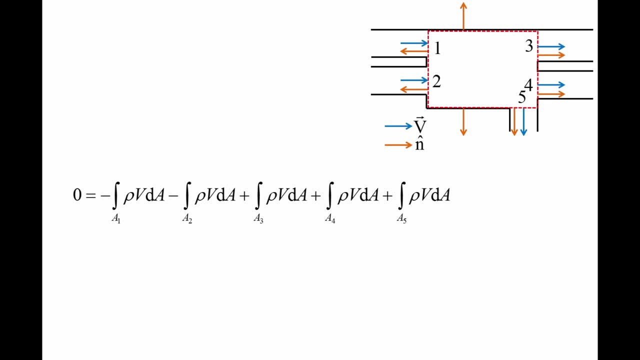 means the dot products for integrals 3,, 4, and 5 become positive. v. The no-slip boundary condition means that the velocity at every wall is 0.. We now have five integrals of density: rho times speed, v times area dA. For most scenarios in fluid mechanics, the density will not vary significantly across a single inlet or outlet, although it may vary between different inlets and outlets. For example, the density at the top and bottom of the fluid will not vary significantly across a single inlet or outlet, although it may vary between different inlets and outlets. 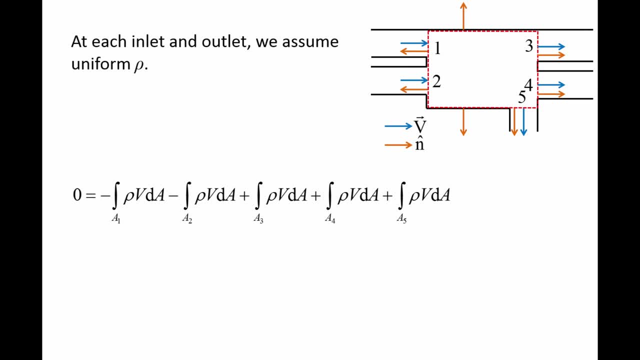 The density at the top and bottom of inlet 1 would be approximately equal, but the density at inlet 1 may differ from the density at inlet 2.. This assumption allows us to remove the density from each integral. We now have five terms that contain the local density, rho times, the integral, v dA. 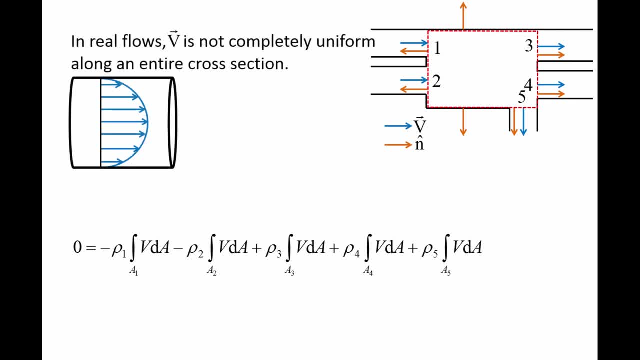 In order to determine the integral of v dA, we would need to know the velocity profile at each inlet and outlet. In real flows the velocity is not completely equal. The velocity is not completely uniform along an entire cross-section. Here we have zoomed in to an arbitrary inlet or outlet. 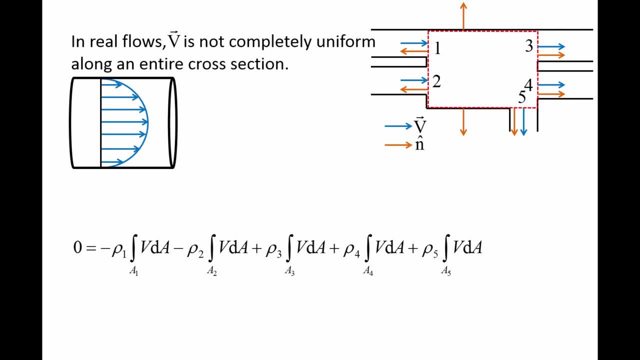 Under certain flow conditions, the velocity profile can be parabolic in shape, with the speed equal to zero at the walls and reaching a maximum at the center, Regardless of the exact flow conditions. v dA integrated over the entire cross-sectional area divided by the total area A, gives the average speed v average for that cross-sectional. 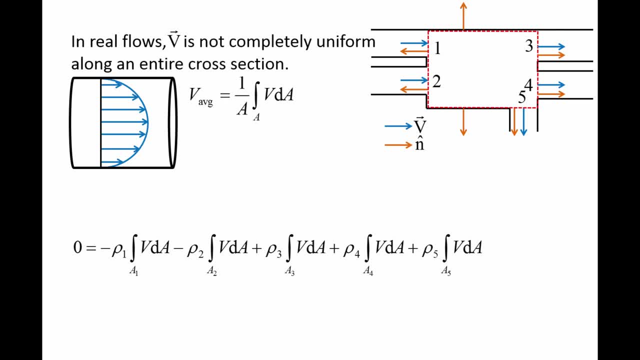 area. Speed times area has the units of volume per time. so v average is the speed of a uniform velocity profile that would produce the same volumetric flow rate as the actual velocity profile. So the integral of v? dA is equal to v average times A. 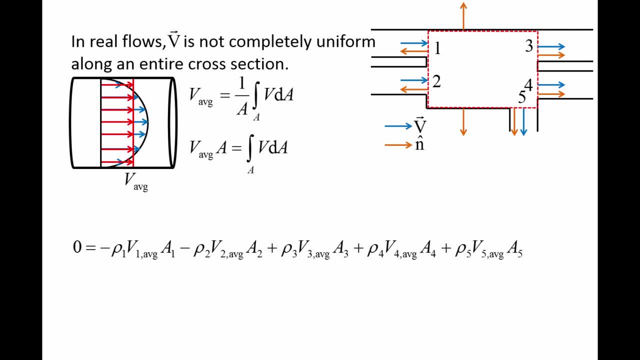 The five integrals have now been simplified to density: rho times the average speed. v average times the area A at each inlet and outlet. Each term has dimensions of mass per time, so the terms represent mass flux rates and will be written as m dot. 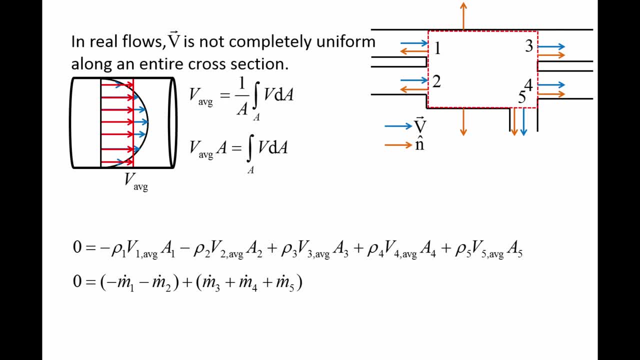 The equation becomes: zero equals negative: m1 dot minus m2 dot plus m3 dot plus m4 dot plus m5 dot. Notice that all terms associated with an inlet are negative, while all terms associated with an outlet are positive. Let's move the two inlet terms to the left side. 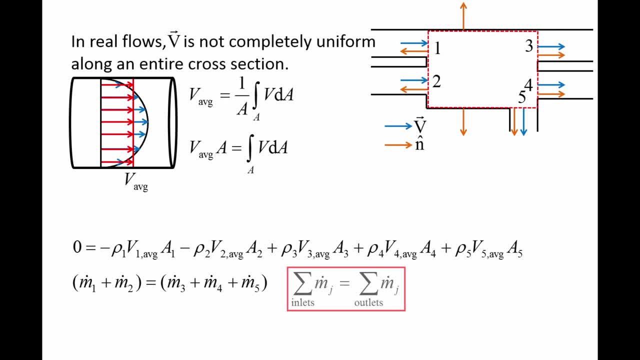 side of the equation. We can write this equation more compactly, as the sum of the mass flux rates through the inlets equals the sum of the mass flux rates through the outlets. The J subscript indicates the inlet or outlet number. This form of the conservation of mass equation. 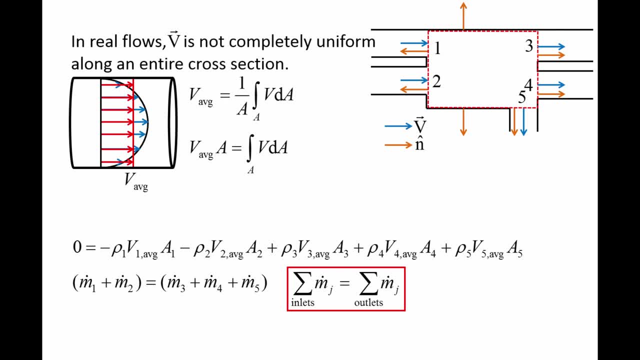 is valid for steady flow through a non-deforming control volume, which represents a wide range of engineering devices. When calculating mass flux rates, it is important to remember that V average is the flow speed as observed from a reference frame attached to the control volume. 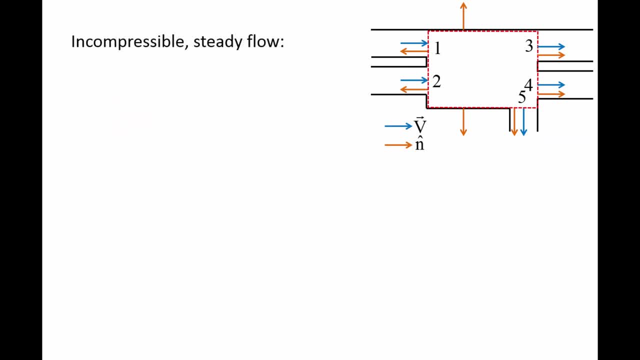 If the density of the fluid at all inlets and outlets are approximately the same, we can further simplify the conservation of mass equation. We start with the conservation of mass equation that we just derived and substitute rho V average a for m dot If the fluid density is the same at all inlets and outlets. 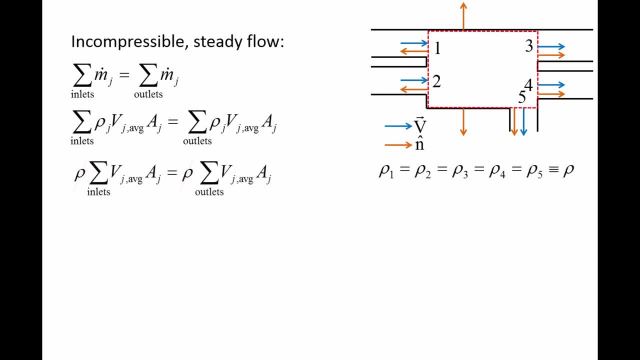 we can remove density from the summations, The densities cancel out and we are left with the sum of V average times a for the inlets equals the sum of V average times a for the outlets. V average times a has dimensions of volume per time. 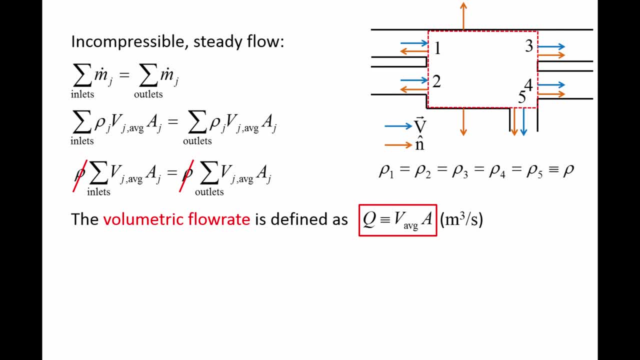 and is called the volumetric flow rate. We will use the symbol q to denote this quantity. The conservation of mass equation then becomes: the sum of the volumetric flow rates at the inlets equals the sum of the volumetric flow rates at the outlets. 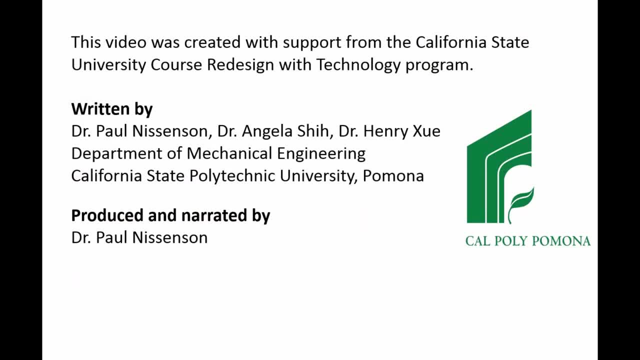 Thetor is surgery at 8 feedback times, q at this. OK, So it's difficult to define the volumetric flow ages under one maximum과 one maximum stage for the inlets and outlets, or inlets under one maximum, So capacity. It's a manipulabilityounivocation. frequency at insulation per unit travel time. kanye Exist of the appropriate characteristics of simple diameter inlets on the position of insulator, The ع, the strength강 seizures at interlocking radius are equal.